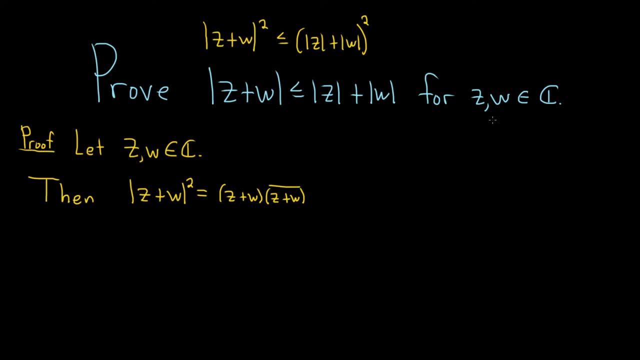 times the conjugate of the complex number, and that's a property which I'll write over here. So I'll do it here. actually, I'll say, since, for any complex number, say u, if you take the complex, if you take the modulus of it and you square it, 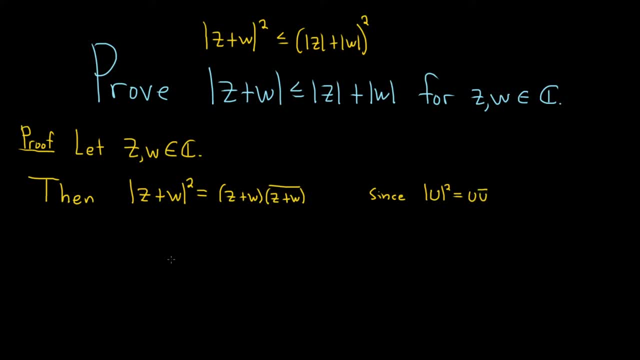 you get u times the conjugate of u. That's true for all complex numbers. That's true for all complex numbers. The next thing we're going to do is well. The next thing we're going to do is well is use the fact that whenever you have a sum like this, 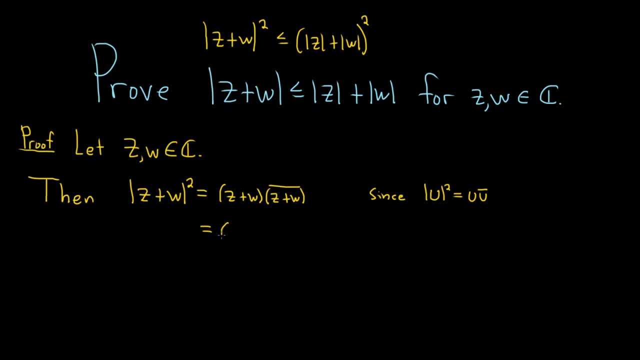 and you're taking the conjugate. you can just take the conjugate of each term, So this would be z plus w times, the conjugate of z plus the conjugate of w, And that's from this property here. I guess I'll say it over here. 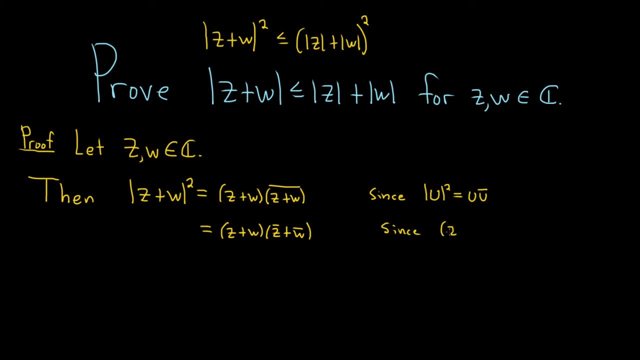 This is since, whenever you have z plus w and you take the conjugate, the conjugate is just going to be the conjugates of the sums. The next step is just going to be regular multiplication. So let's go ahead and multiply. So we're going to distribute. 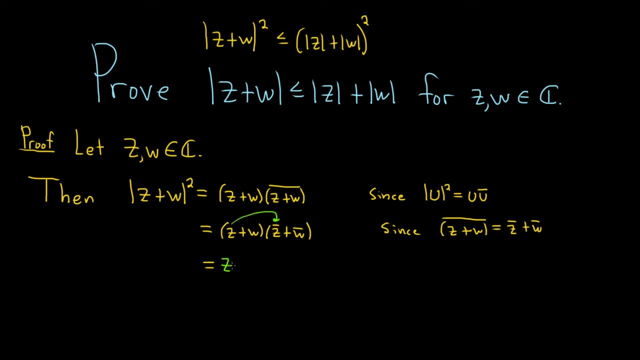 So we have z times z conjugate, So z times z conjugate And then z times w conjugate. So z times w conjugate And then w Times z conjugate And then w times w conjugate, Just like that. 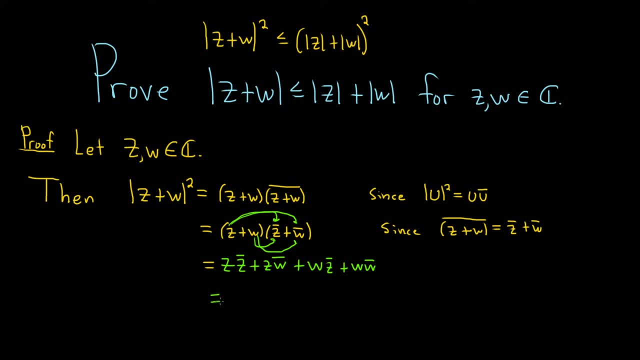 All right, Now we can use a property that we already used. We can use this one again twice, So this will be the modulus of z squared. I'm going to rewrite this. I'm going to just keep this one the same Z. 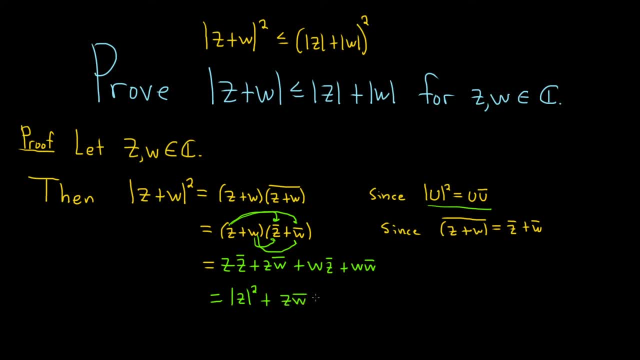 W conjugate. And then this one: I'm just going to put the z in the front. Okay, This is just by commutivity. So z conjugate, w, Like that. And then on this last one, we'll use that rule again. 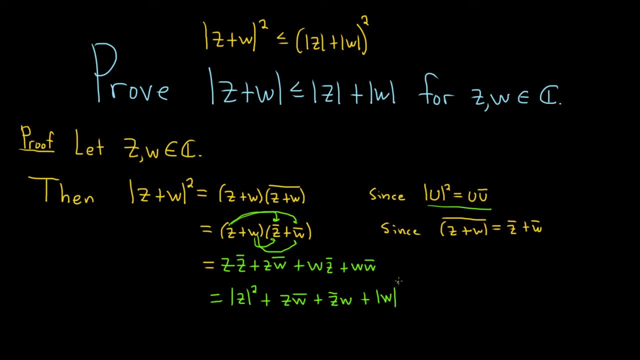 that a complex number times its conjugate is the modulus squared. So this is since We did two things here. So since you know, whenever you have the modulus of a complex number squared, it's the complex number times the conjugate. 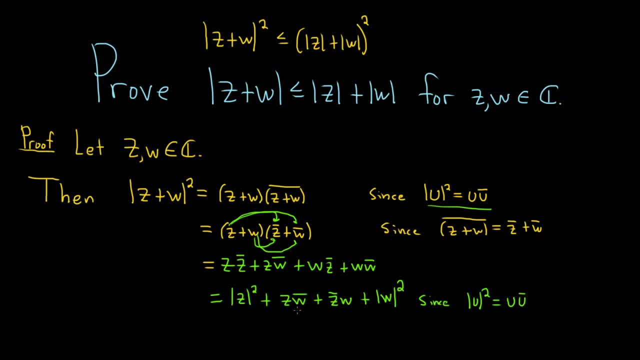 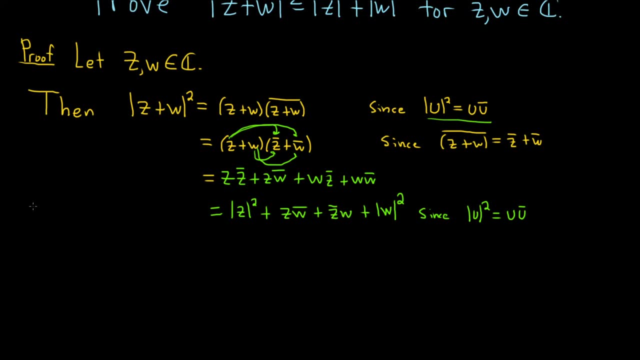 And we also use commutivity. I won't write it, But multiplication of Complex numbers is commutative. Now we somehow want to use another identity. So there's something that tells us that the real part, or two times the real part, 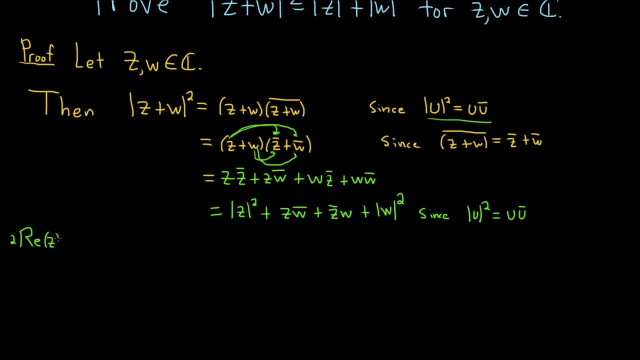 of a complex number, z is equal to the complex number plus the conjugate of the complex number. Okay, So here we need to somehow Write this inner term, These inner terms here, as a complex number and its conjugate. So I'm thinking, let's do it in steps. 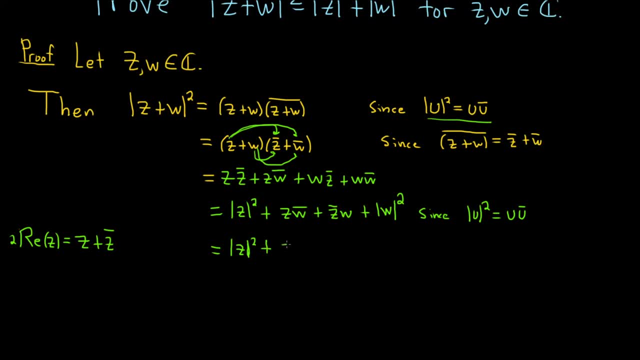 Let's start by just putting two bars above the z, like this: So bar bar. It's the same thing, right? Because if you take the conjugate, of the conjugate, you get the original thing. So let me just write the rest of it here. 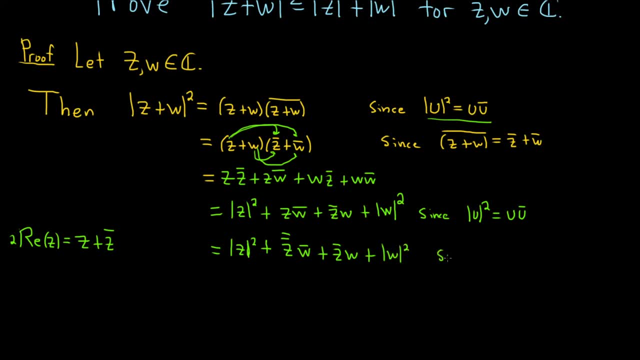 And then plus the modulus squared. And this is since the conjugate of the conjugate is the original, So c, If you have a complex number u, you take the conjugate of the conjugate, you just get the regular thing. And now we're going to use another property. 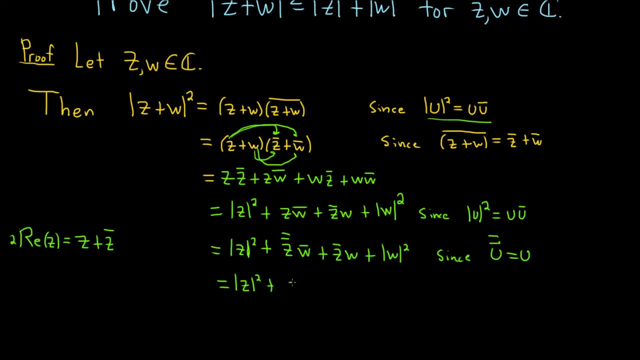 So now what we can do is, we can just do this: We can write this as z conjugate w and then conjugate, And the conjugate basically distributes over the multiplications. We get conjugate, conjugate and then conjugate. So and then plus z conjugate w, plus. 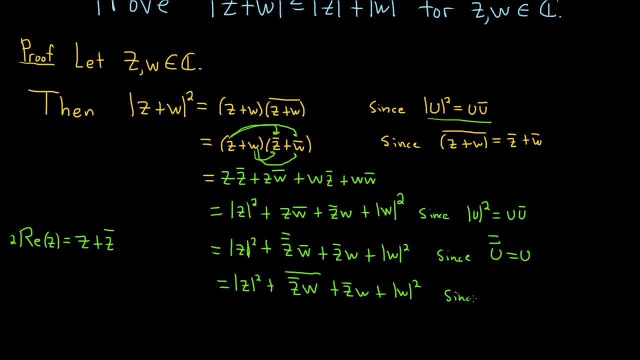 The modulus of w squared. And this is since, if you have, you know the conjugate of a product, it's the product of the conjugates. Okay, You can do that. So, and you know this formula over here on the left, you know you could write it like this: 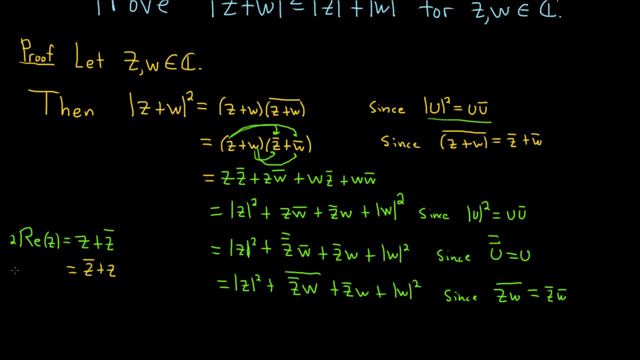 because, you know, the addition is commutative. That's basically what we have here now We have. this is our z here You see it, That's the same thing as as this here. So now this is going to be the modulus squared plus two times the real part. 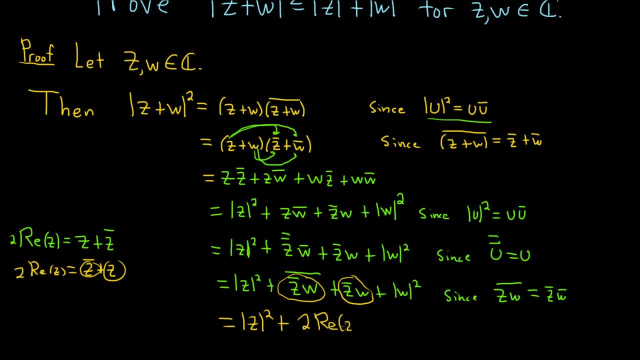 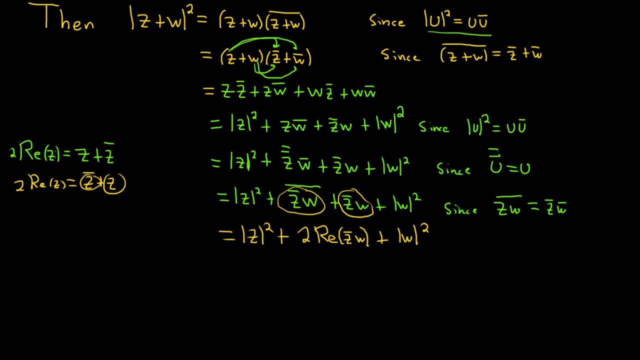 Two times the real part of the conjugate of z, times w plus the modulus squared: Okay, Times plus the modulus squared: All right, And that's because of this one here, this one over here. So I'll just write, since, Since two times the real part of z, 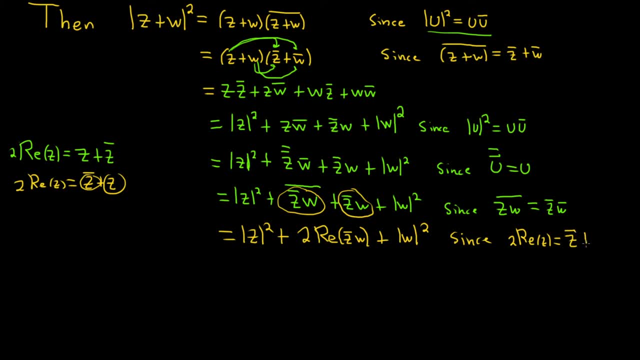 Trying to show a lot of work here. Conjugate of z plus z, Trying to be really, really thorough. So this is equal to, or this is less than, or equal to, the modulus of z squared. So the the real part of a complex number, z. 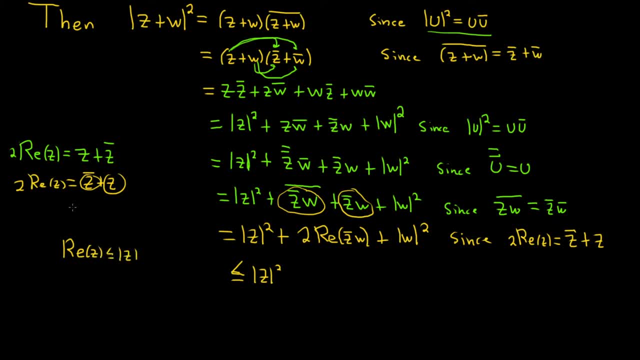 If you think about it, It's less than or equal to than, or equal to the modulus of z. I mean, if you think about it, if you have, z equals x plus iy, right, so the real part of z is x and you can say that. that's you know. 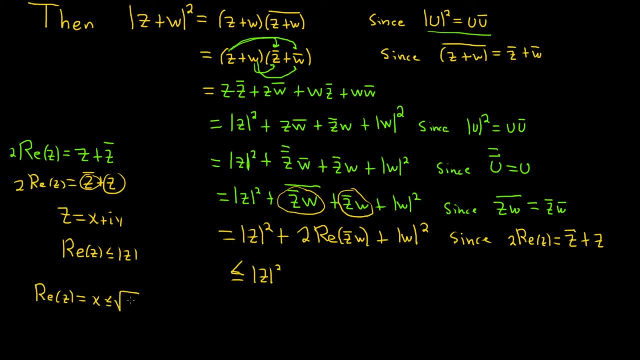 less than or equal to the square root of x squared, which is less than or equal to the square root of x squared plus y squared, which is the modulus of z, So the real part of a complex number. actually, you could say it's equal here, If it's positive, I guess. 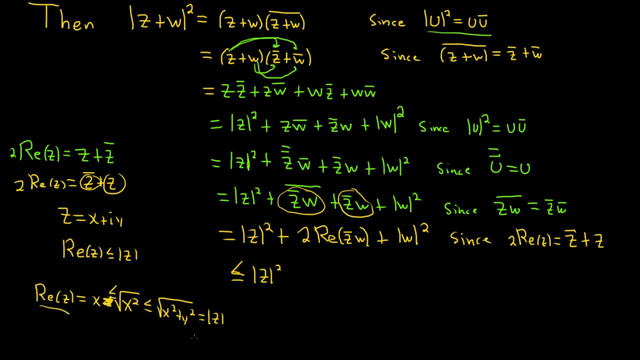 I'll just say less than or equal to. So this is less than or equal to the modulus of z. So this is plus two, and then modulus of z conjugate, w plus modulus squared, And this is since the real part of a complex number. z is less than or equal to the modulus of. 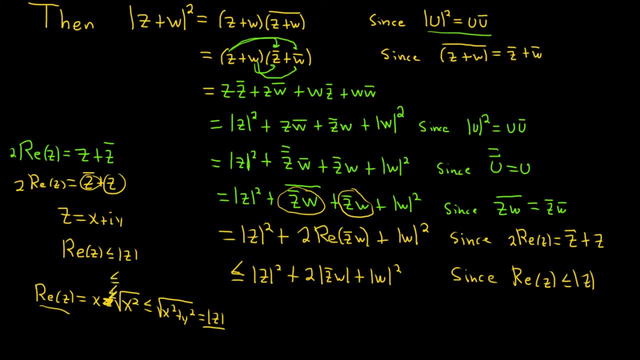 z. It's a really, really short proof there. It should be a less than or equal to there, Sorry, Okay, So now we can do this: This is the modulus of z squared plus two, and then you can break this up. And you can do this because if you have the modulus of a product, that's 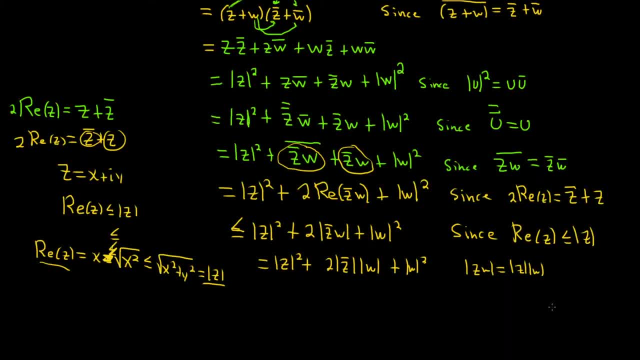 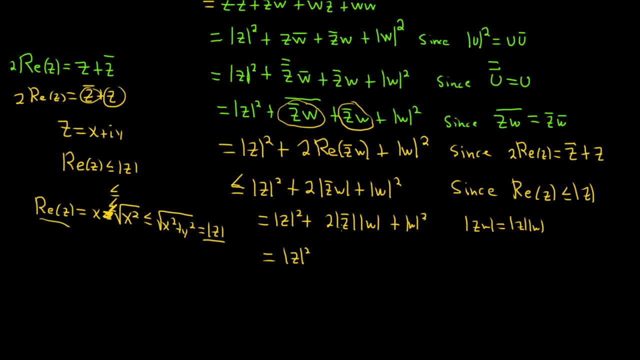 the product of the moduluses. Okay, And whenever you take the modulus of a product, you can take the modulus of the conjugate. That's the same thing as the modulus of the regular complex number without the conjugate. Okay, That's another property, A lot of properties.